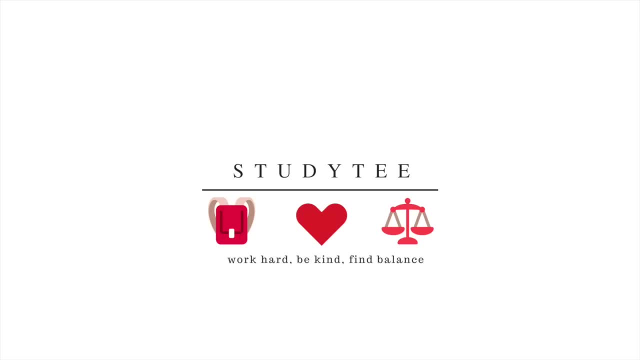 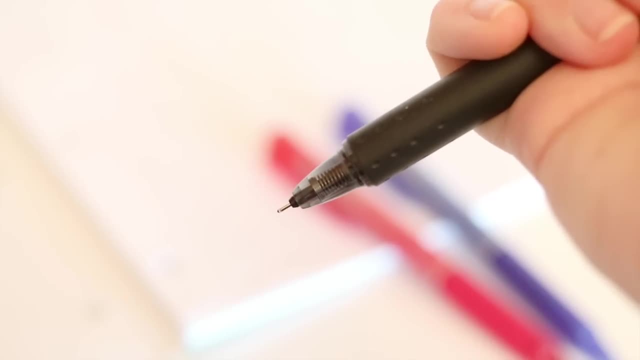 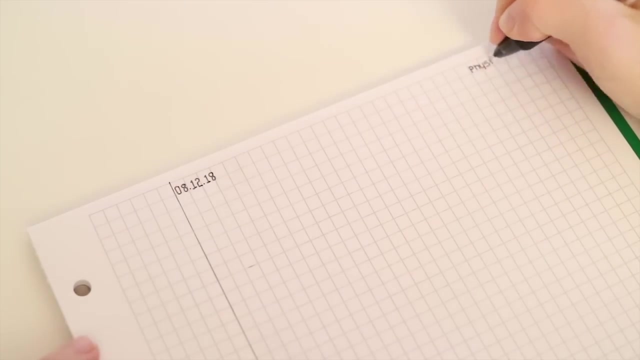 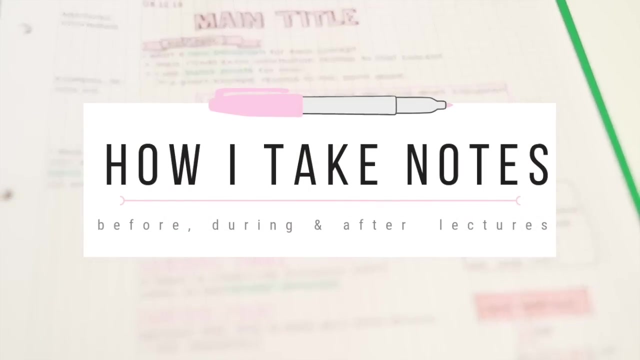 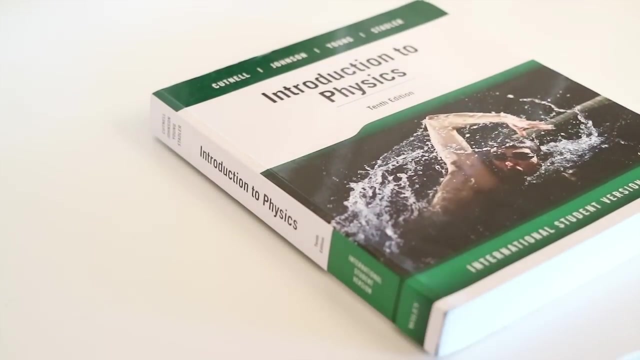 Hello everyone. I think it's safe to say: long time no see, but I'm finally back with a new video. Today I'm going to make an updated video on how I take notes, and this is going to be a combination of both lecture notes and textbook notes. During my first semester of 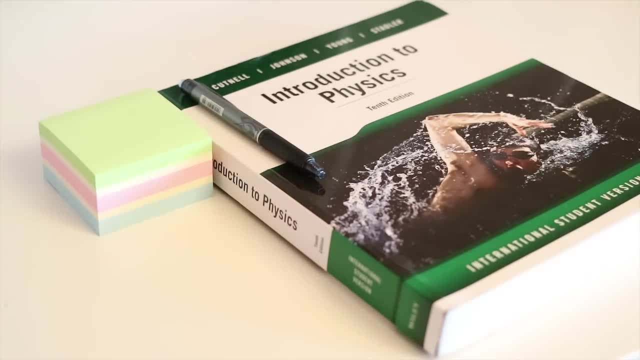 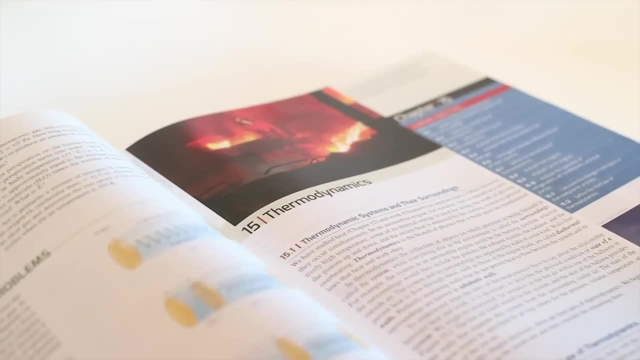 university, I've tried out different techniques for note-taking and I've finally found the way that works best for me. So I'm going to share some of the tips that have helped me take notes that are both efficient and neat, and I hope that they can help you as well. For me, my note-taking. 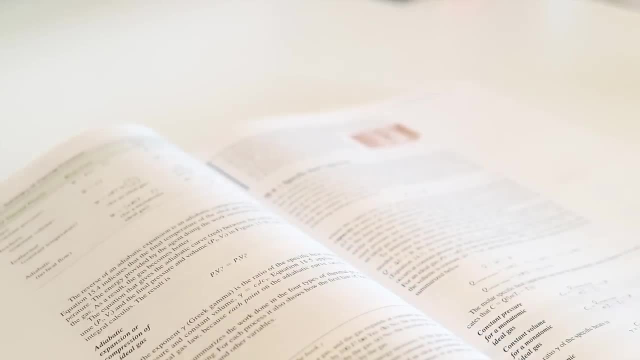 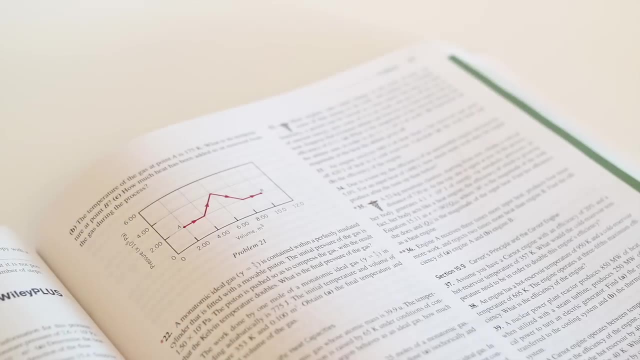 process starts the day before the lecture. The first thing I do is that I quickly skim through the topics for the upcoming lecture, and this is just to get an overview of what I'm going to learn, so that I'm a bit more prepared. Once I've skimmed through the pages, I like to just write down some. 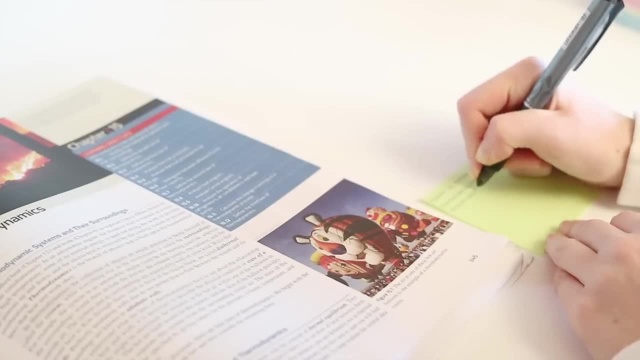 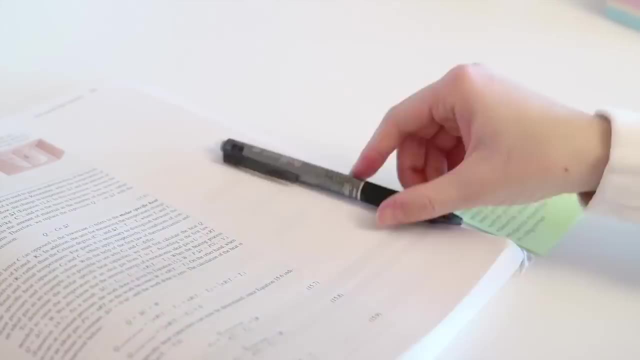 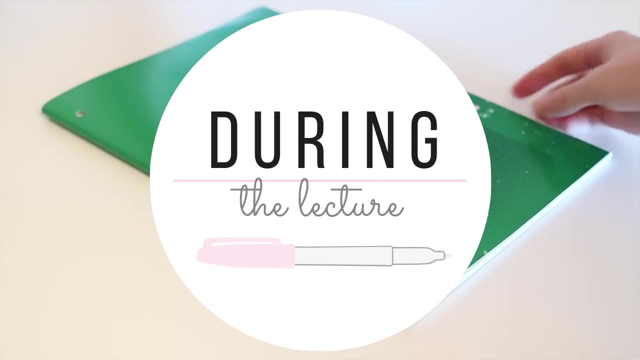 keywords on a piece of paper. This is going to be my checklist for later, to make sure I've included all of the central topics and concepts in my notes once they're finished. During lectures, I prefer using grid paper for my notes. I feel like the grid is a big support. 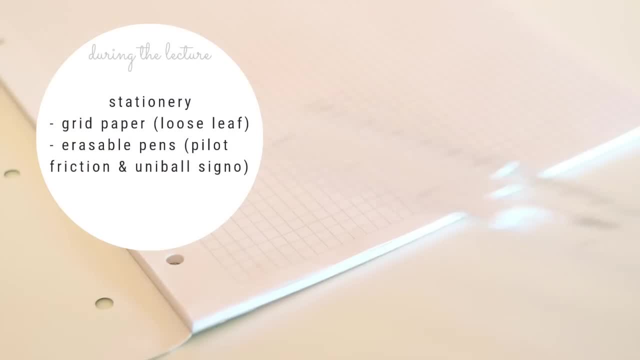 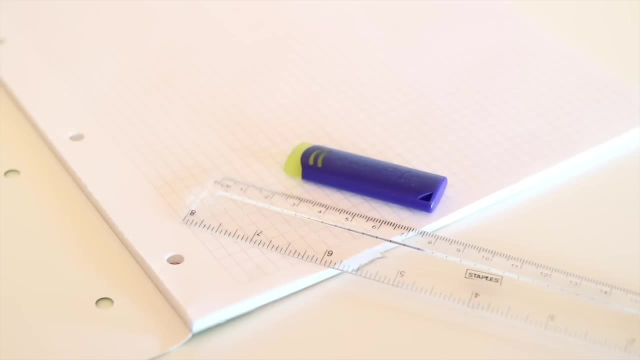 when it comes to making my notes neat and organized, and it also makes the spacing between lines more narrow, which is useful for those of us with small handwriting. I also prefer loose-leaf paper over notebooks, just because I don't have to deal with the spiral getting in the 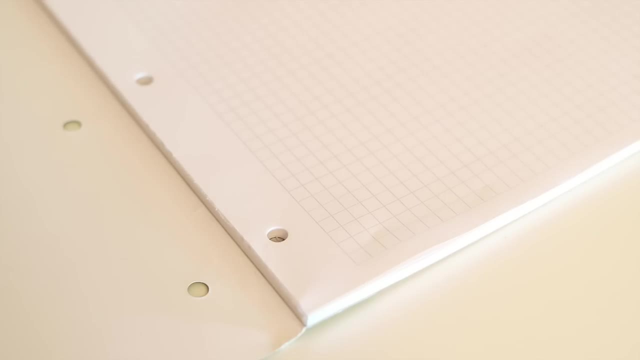 way, and also because I put my notes in a binder when they're finished. When I first started teaching, I started by writing down the topics that I wanted to learn, and then I started writing down the topics that I wanted to learn, and then I started writing down the topics that I wanted to learn. 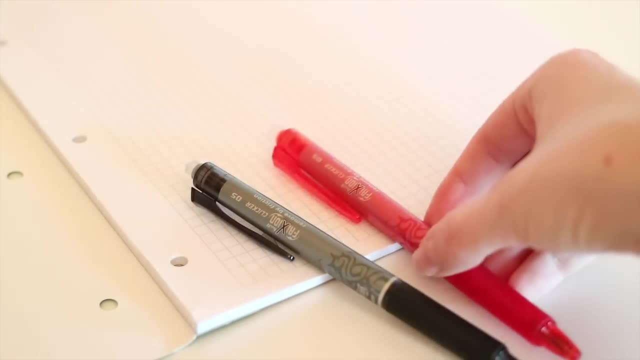 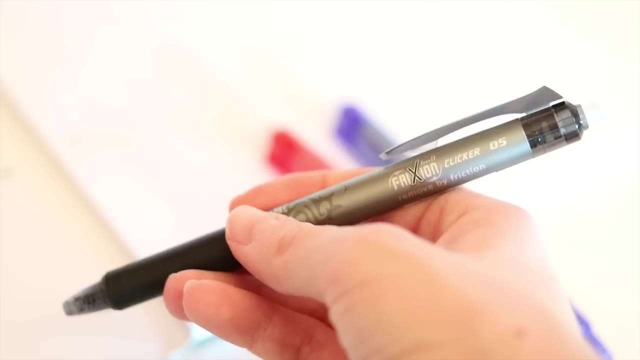 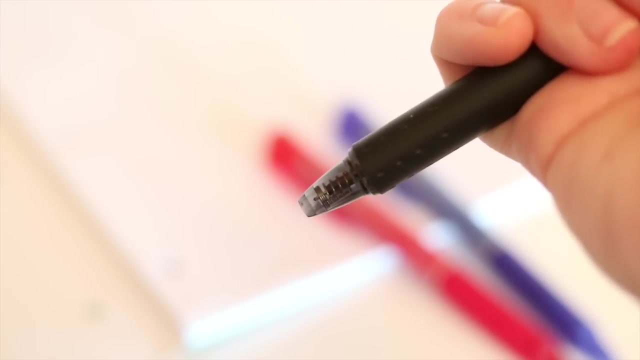 When it comes to stationery, lately I've been mostly using erasable pens. That way I don't have to cross over or use white out on any mistakes and I can also just change my notes as much as I like. The pens I use the most are the Pilot FriXion 0.5mm pens for writing, then the thicker Pilot. 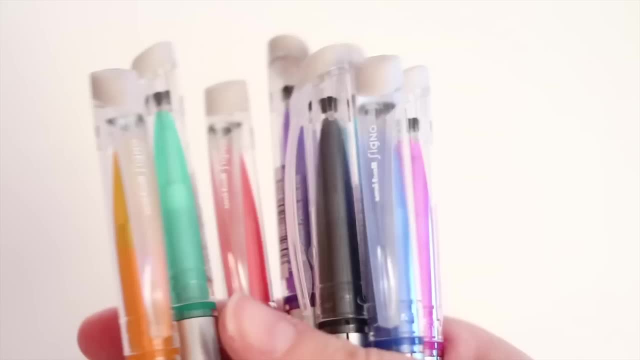 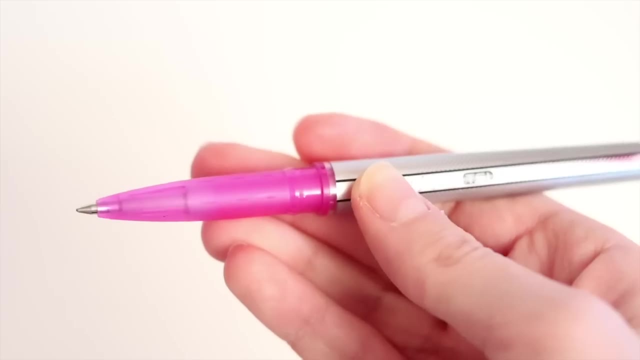 FriXion pens for coloring and the Uniball Signo erasable pens for some extra colors. You should keep in mind that these pens may be erased by friction, heat and other things, but if you are a bit careful you shouldn't have too much trouble with them. 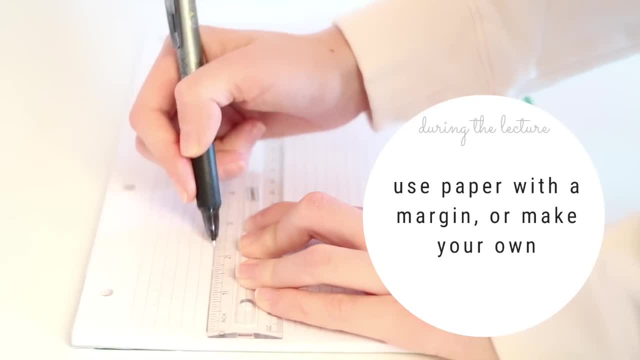 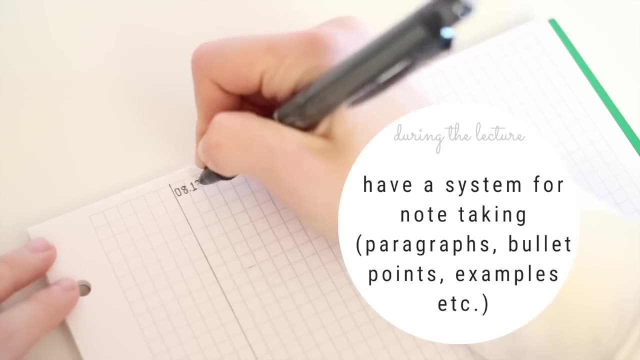 If there isn't already a margin on the paper I use, I'll quickly make one before I start writing, just to get some extra space that I will use later. A good tip for keeping your notes neat and organized is to have a certain system for. 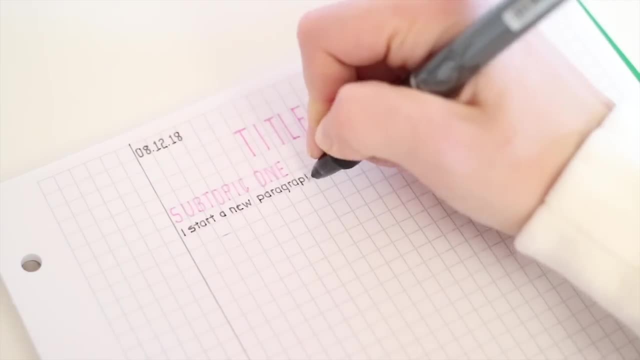 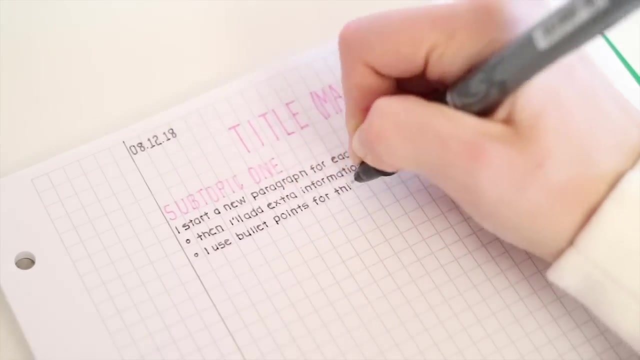 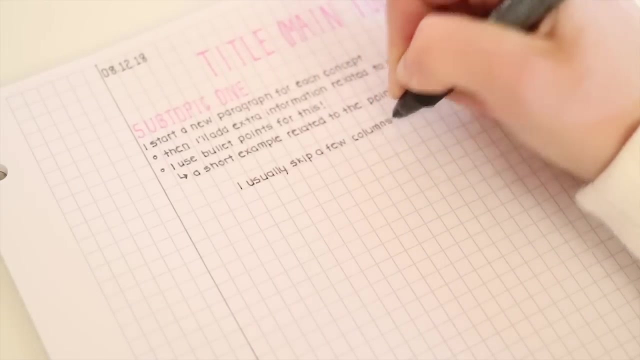 organizing what you write that you stick to. For example, I start a new paragraph for each concept, Then I use bullet points to add extra information related to that concept and I use arrows to include short examples related to the current topic. I also write any calculation examples in a box towards the middle of the page, which 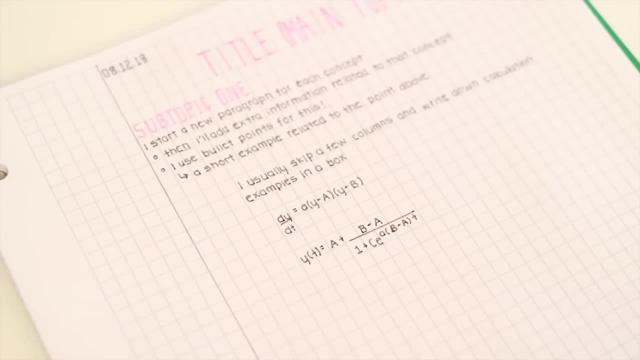 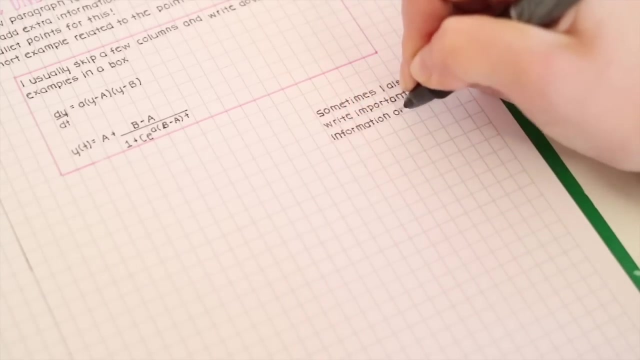 lets me find them easily if I go through my notes at a later point looking for a particular calculation. I also use these kind of cloud boxes to include any additional important information that doesn't necessarily fit into one of the paragraphs. My point isn't that you should try to copy this particular note-taking system, but that 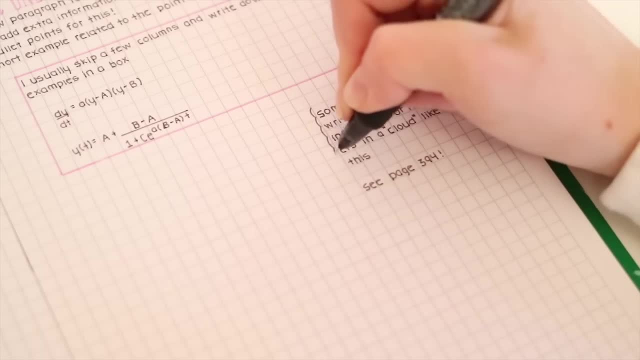 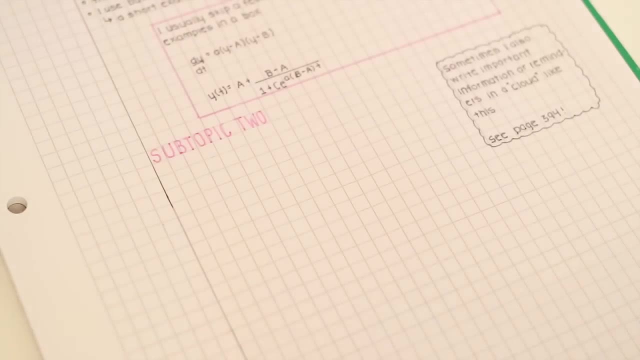 you find one that works for you. Having a system helps you in keeping your notes organized, and you also spend less time figuring out the layout of your notes. Another thing that I've been doing for a while is using a colored pen to write down. 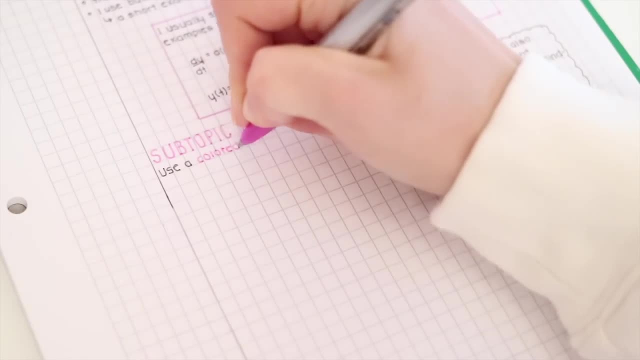 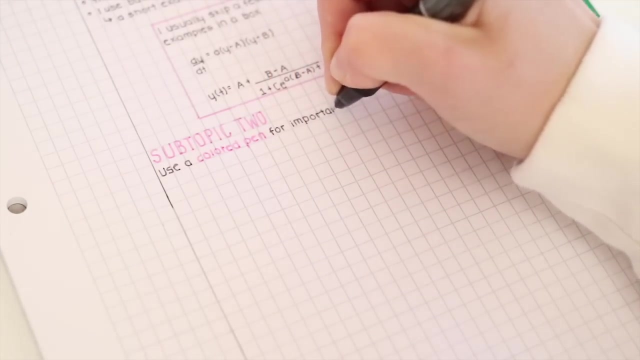 important terms. When I skim through my notes later while revising them, I can easily see the most important terms, and I also feel like the process of changing pens and taking a bit of extra time to write down these terms helps me in remembering them. 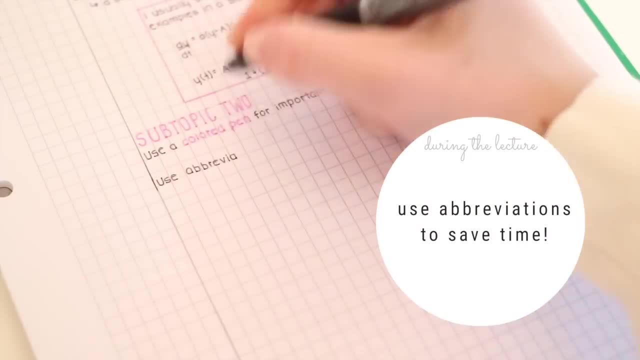 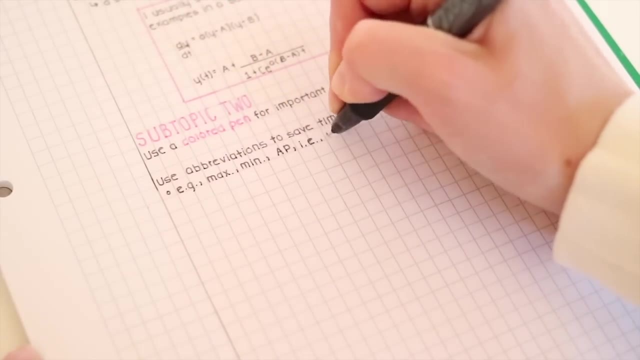 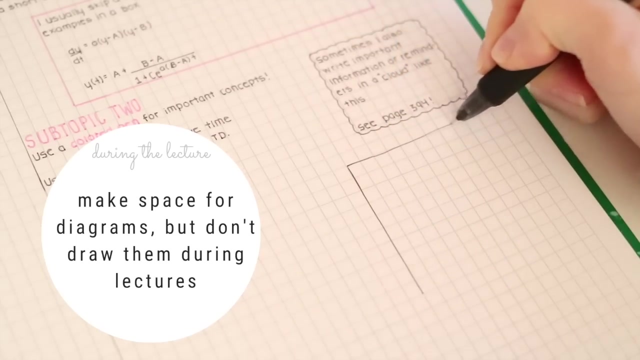 Another tip to save time while taking notes is to use abbreviations as much as you can. Just make sure that you remember what the abbreviations mean, so that you don't get confused while looking through your notes later. A final thing that I've found to be very useful during lectures is to make space for diagrams. 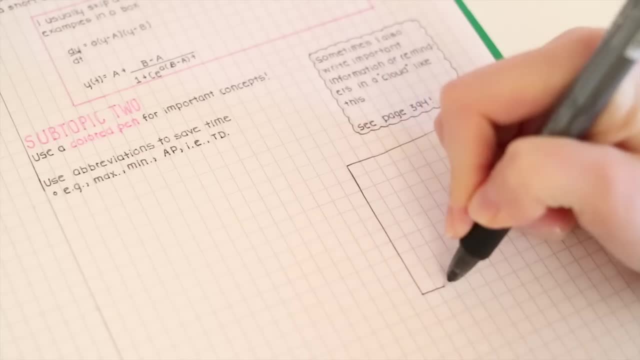 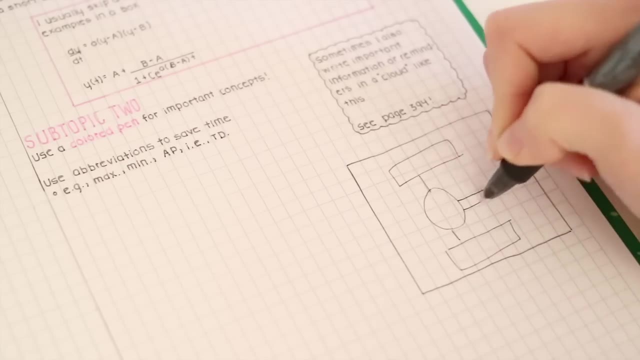 that the professor goes through, but waiting to draw them until after the lecture. As you may know, diagrams is one of the most important things in a lecture. It's one of the most important things in a lecture. It's one of the things that I learn the most from and therefore a central part of. 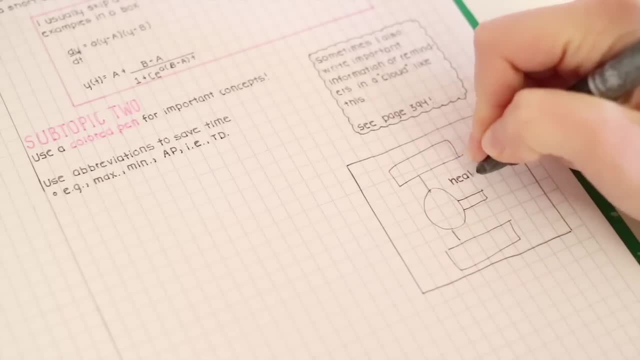 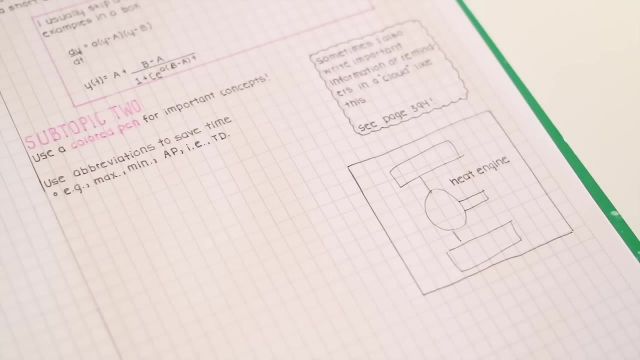 my notes and I've found that by drawing them when the lecture is over lets me make them more detailed so I can learn more from them, while I also get to revise the topic. while drawing the diagrams, I usually return to my lecture notes either later the same day or the day after the lecture. 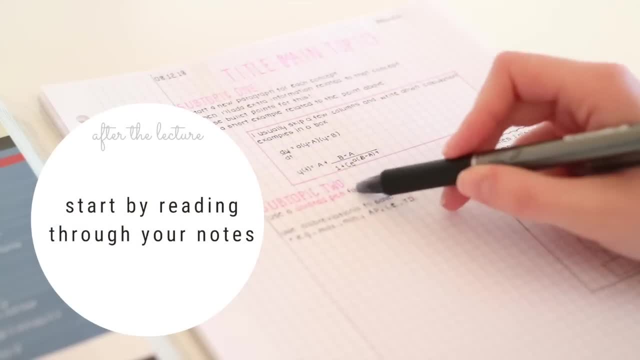 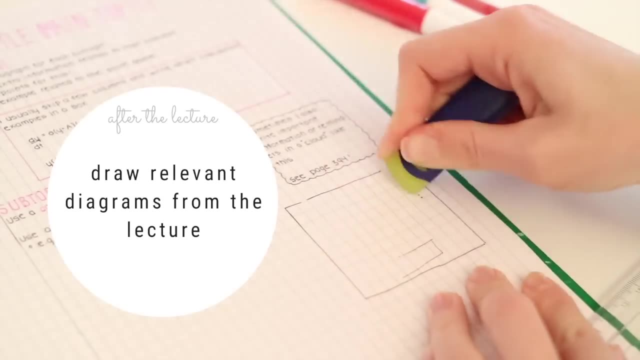 I start by quickly reading through them so that I remember the topic well before I continue working on them. The first thing I'll do is to draw the diagrams we went through during the lecture. Drawing them at home means that I can spend more time making them detailed and understandable. 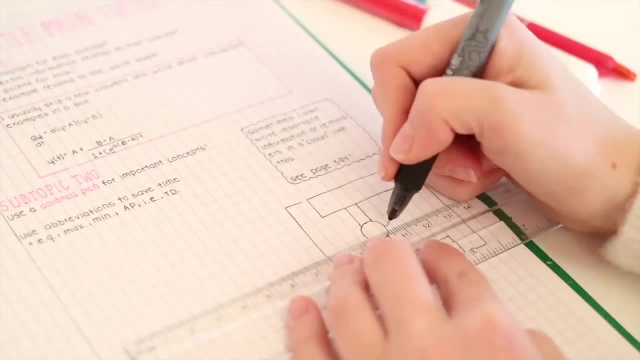 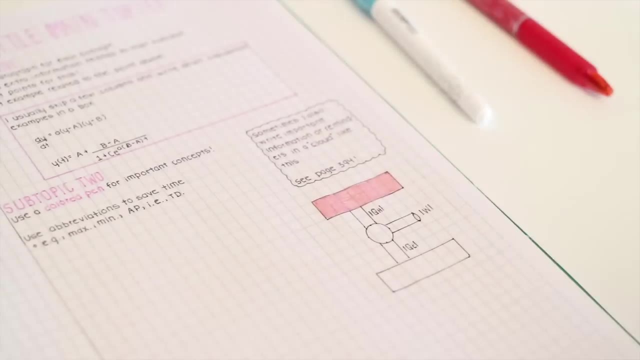 and I also know that I'm only spending time on diagrams that are directly relevant to the topics we've actually learned about. If I find that there are other diagrams from the textbook that are relevant, I will, of course, draw them as well, but most of the time I've just used the ones that my professors 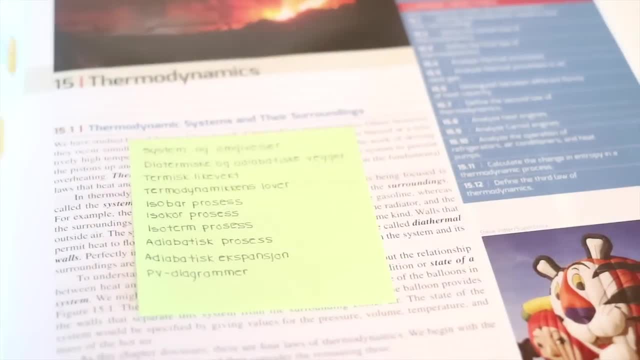 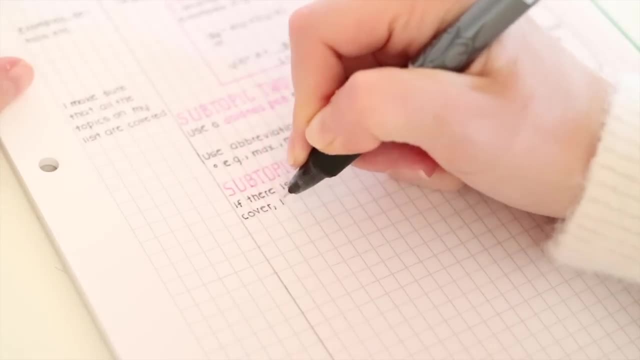 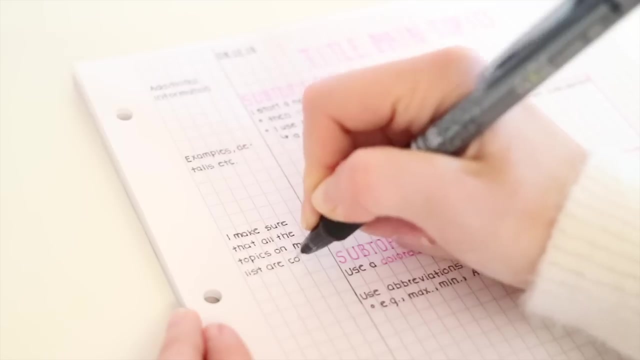 have used, Then I will return to the checklist I made in the beginning and see if we've covered all the central topics. If we're missing anything, I'll add it to my notes and I also use the margin to add any additional important information, more examples or any details that I feel is important. 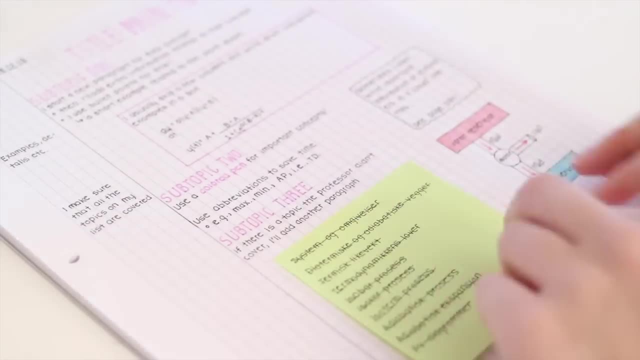 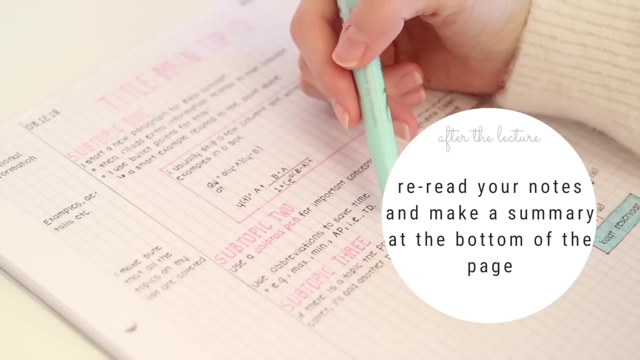 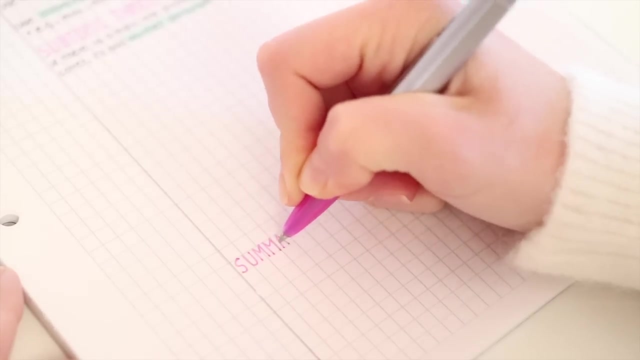 to include. After this, I will read through my notes once again, and I sometimes use a highlighter for this step to highlight what I feel are the most important points in my notes. The last thing I'll do is that I will write a brief summary of what I've learned during. 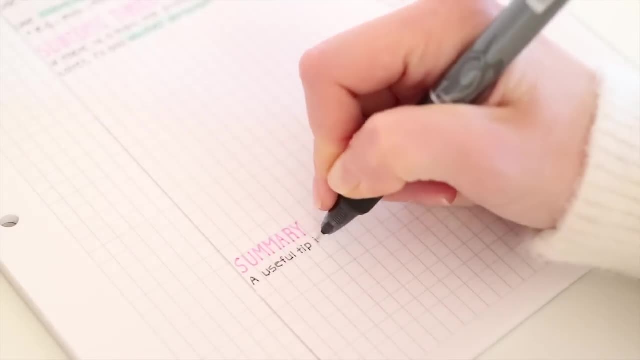 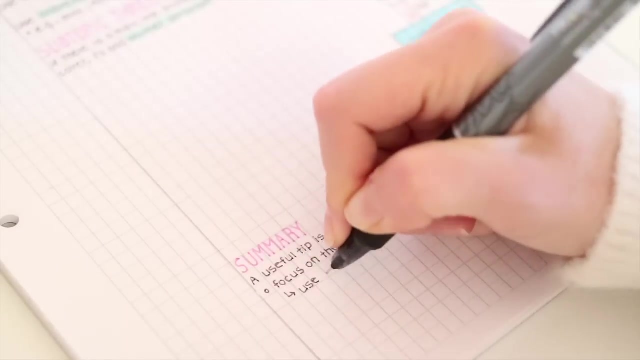 the lecture, I'll write a brief summary at the bottom of the page, where I focus on the main ideas and also the concepts I've found to be the most difficult ones, and then I can use the summary when I want to quickly revise my notes before a test or an exam. 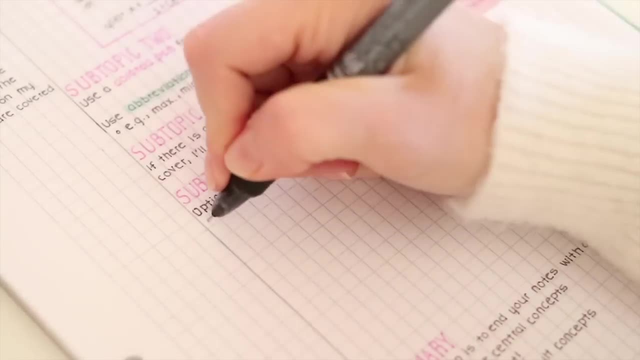 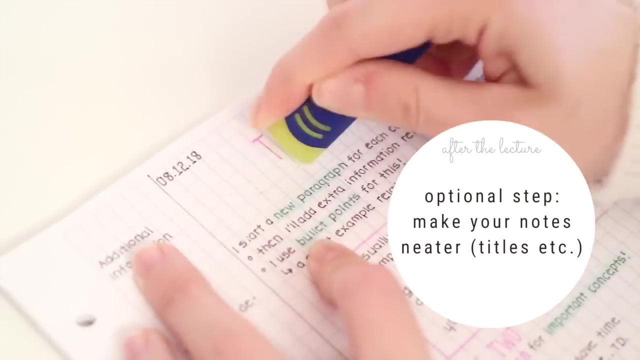 Finally, a completely optional last step is to take a couple of minutes to make your notes look neater, if you feel like it. I usually don't do this myself, but if my notes look especially messy or if I just want to do something creative during a study break, I'll write a brief summary. 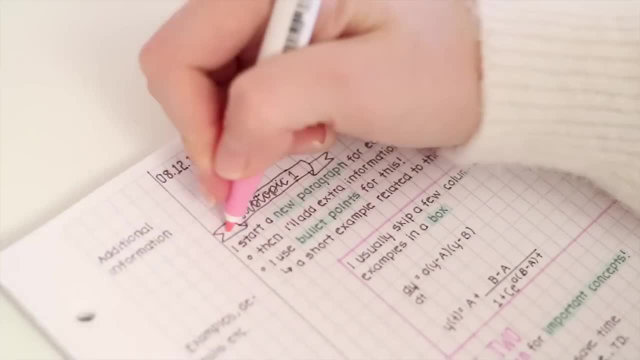 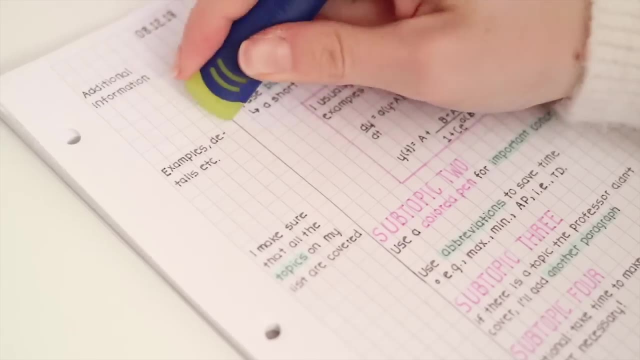 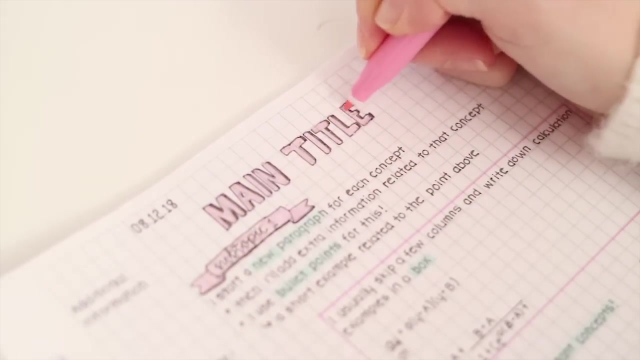 I might change the title, make the subheadings a bit fancier, or just anything that makes my notes more appealing to study later. This is, of course, not necessary, though, and if you don't feel like doing it, you definitely should not feel like you have to.